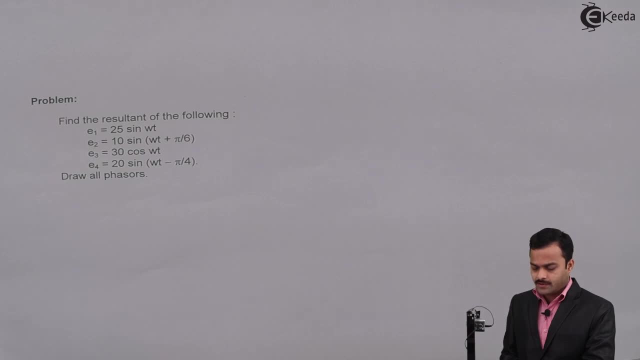 all of them are voltages. E1 is given as 25 sin omega t, E2, 10 sin omega t plus pi by 6, E3, 30 cos omega t and E4 20 sin omega t minus pi by 4.. We are supposed to find out. 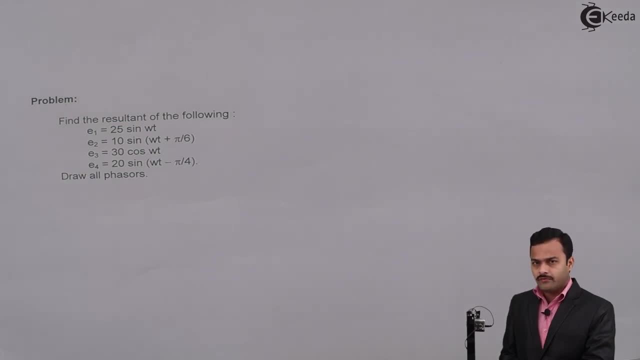 the resultant and we have to draw all phasors. So how to start? One thing you have to keep in mind: All these are the equations of a state, Standard sinusoidal waveform. So first step, we have to compare these equations with standard. 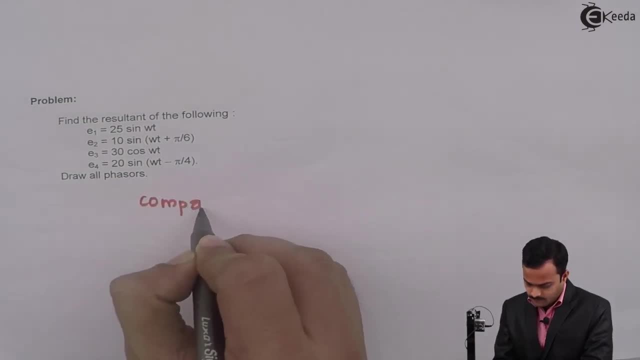 sinusoidal waveform. So I am comparing with E equal to Em, sin omega t plus pi. Make sure that all the waveforms our equations given are from a state should have this form: sin omega t plus 5.. So if I compare first equation I will get: 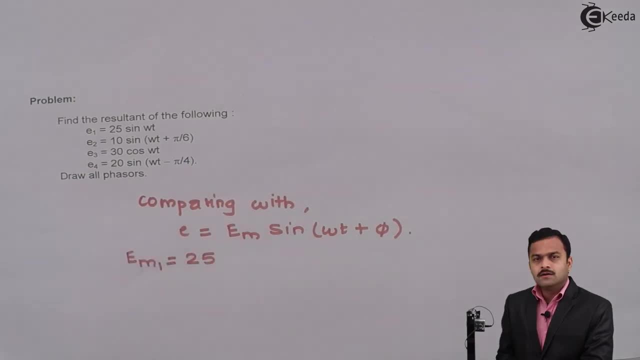 E, m 1, 25 and phi 1 is 0 degree. So I can say E 1 can be represented as 25 at an angle 0 volt. So what I have done, So what I have done, From the equation I got a phasor form. Similarly, E 2 I can write directly: It is 10 at an angle. 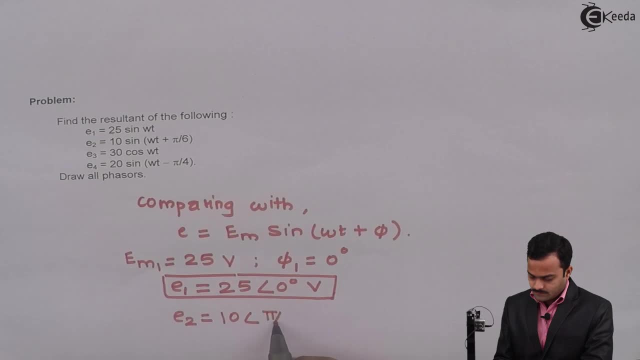 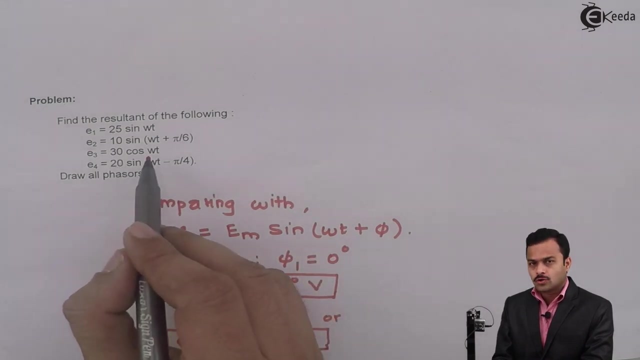 pi by 6 radian. Let us convert that into a degree. So E 2 is nothing but 10 at an angle 30 degree. I cannot compare E 3 directly with this standard equation. Why? Because in standard equation it is sin and here it is cos. 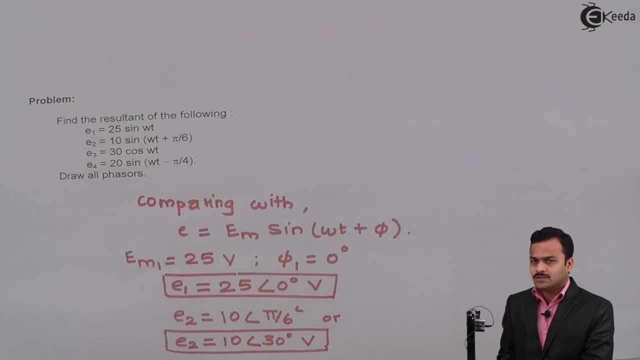 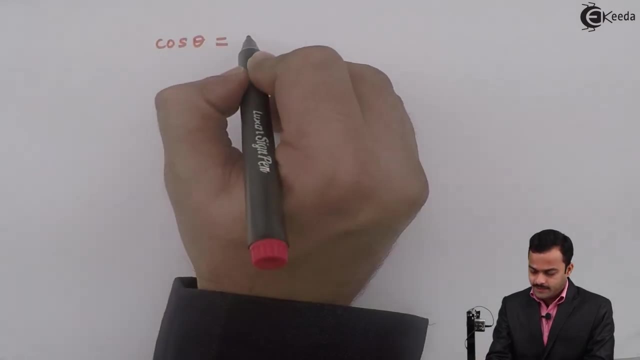 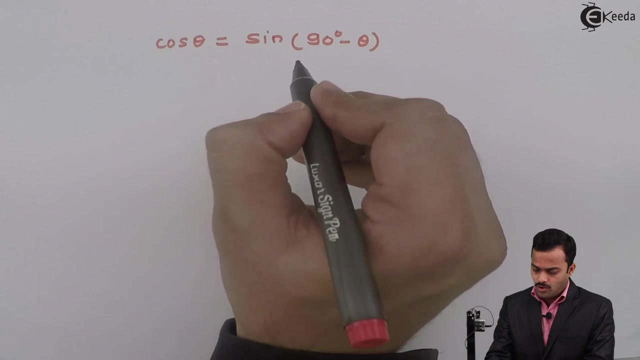 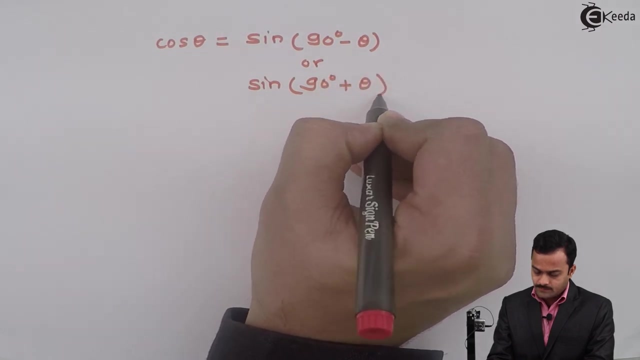 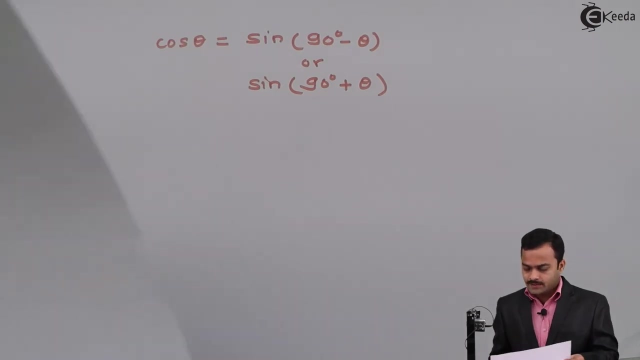 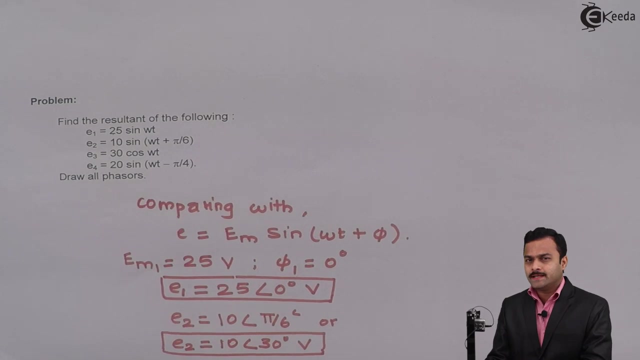 So I need to convert this cos into sin. So the formula is cos theta can be written sin 90 minus theta or sin 90 plus theta, Which one we will take. How to decide. Whenever I use a formula for cos to sin conversion, I have to make sure that theta should remain positive. Why? 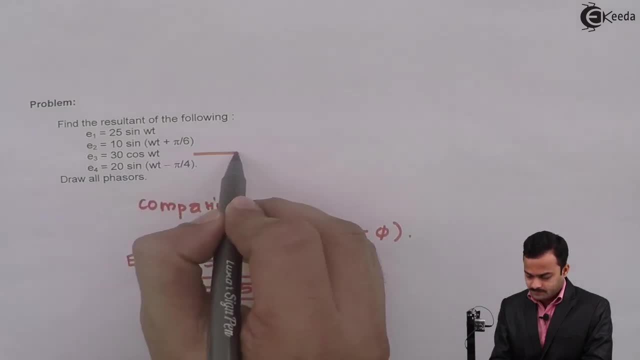 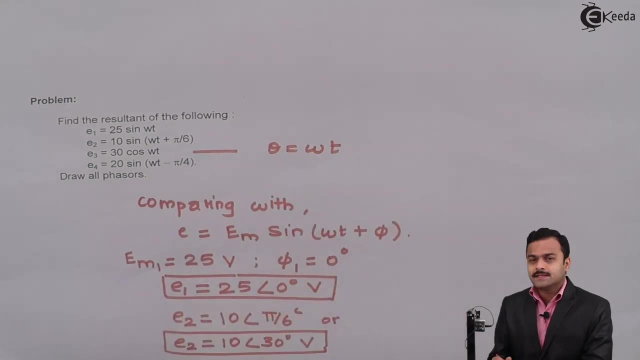 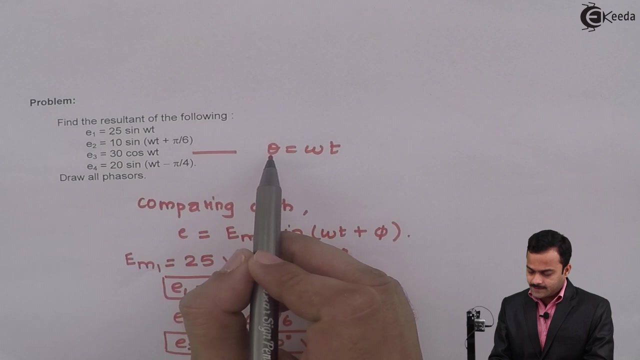 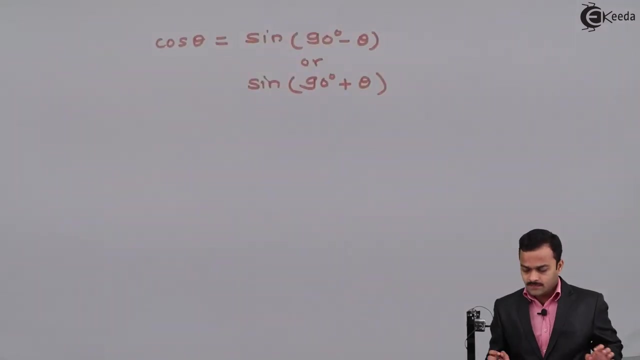 Because theta means omega t over here and this is a frequency. So in a standard equation omega t is always remains positive. So whenever I am to convert cosine into sine, I have to make sure that this omega t term should remain positive. Hence I will use second formula. So the e 3 is given as 30. 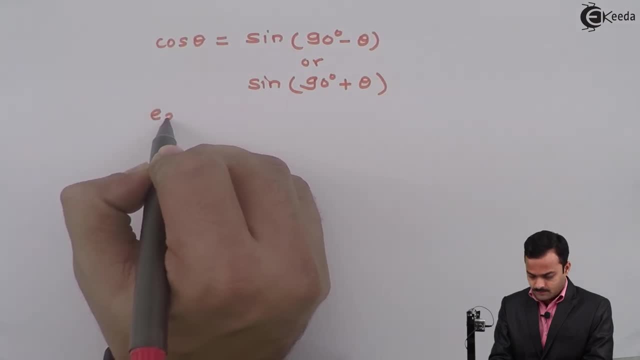 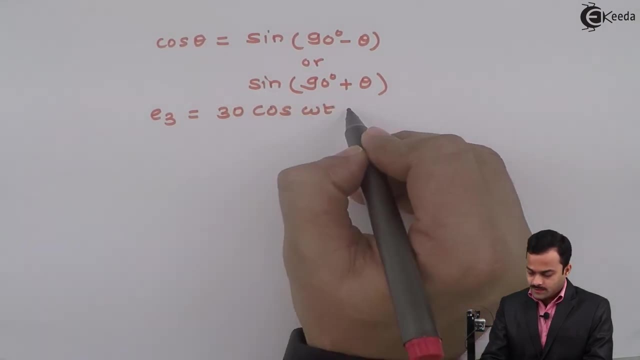 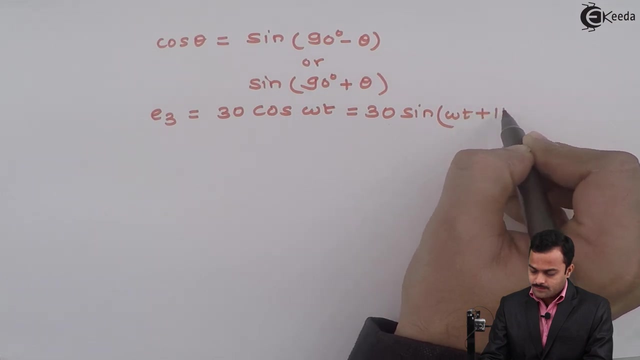 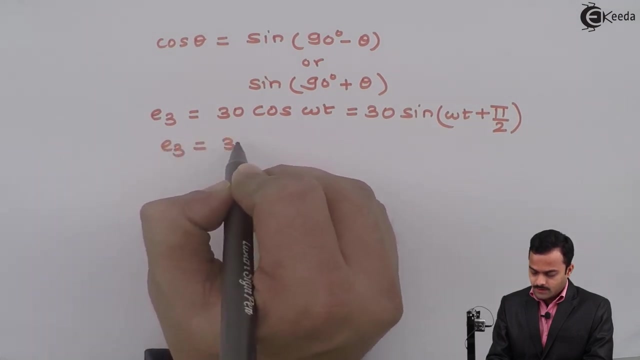 cos omega t, which is nothing but 30 sin omega t plus pi by 2.. So that I will get e 3 as 30 at an angle pi by 2 radian. Or e 3 is 30 at an angle 90 degree volt And e 4 is given as 20 sin omega t minus. 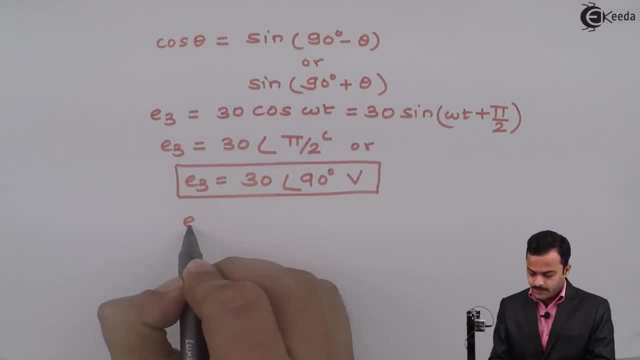 pi by 4.. Simple comparison will give me e 4 as 20 at an angle minus pi by 4 sin omega t, radian, Or in degree it will be 20 at an angle minus 45 degree volt. Now, considering all these equations, if I want to get a resultant, it will be very difficult. 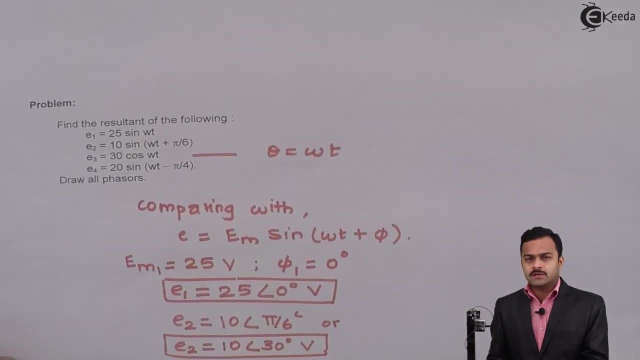 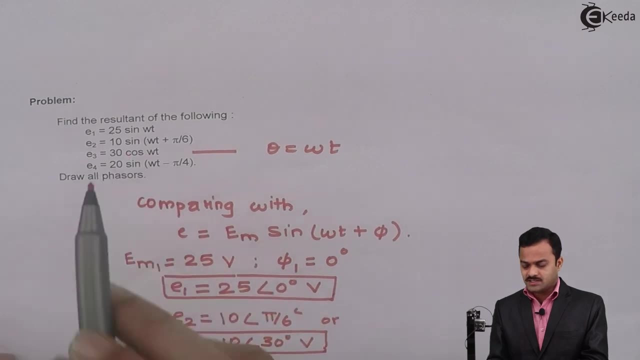 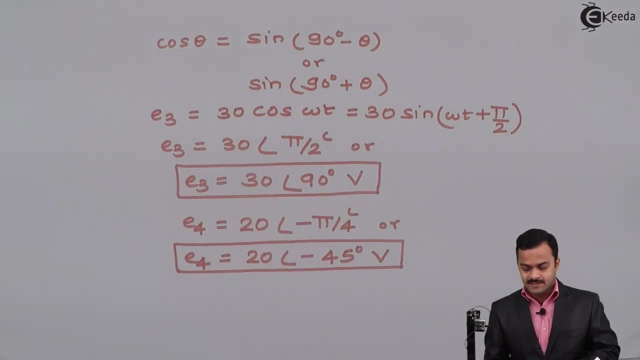 problem because every time I have to use sin to cos conversion or may be a factorization instead. what I have done, all the waveforms, equations I converted into phasors And these phasors I am going to insert in calculator to get a resultant. So resultant emf er is: 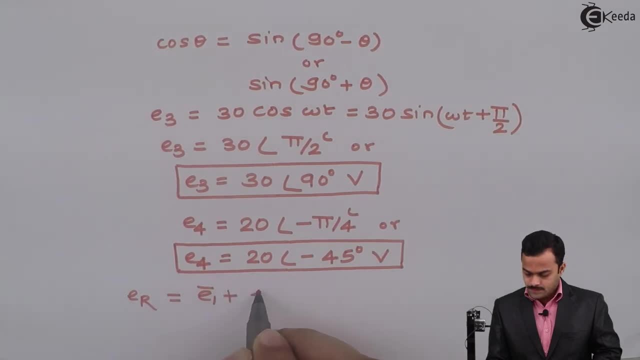 e 1 bar plus e 2 bar plus, e 3 bar plus e 4 bar Bar indicates it is a vector quantity having a magnitude along with the angle. So let us write what is e 1.. So e 1 we have calculated as 25 at an angle 0, e 2, 10 at an angle 30,. 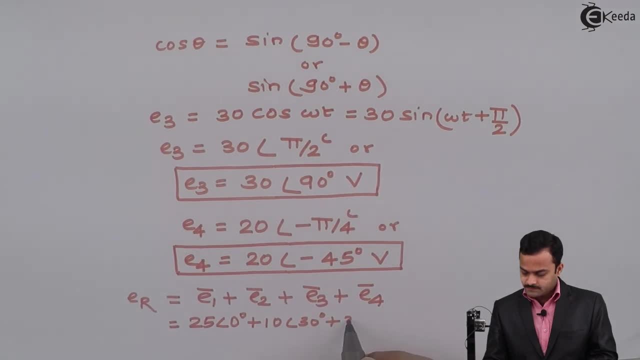 e 3: 30 at an angle 30. So we have calculated as 25 at an angle 0, e 2: 10 at an angle 30, e 3: 30 at an angle 90 and e 4: 20 at an angle minus 45 degree. 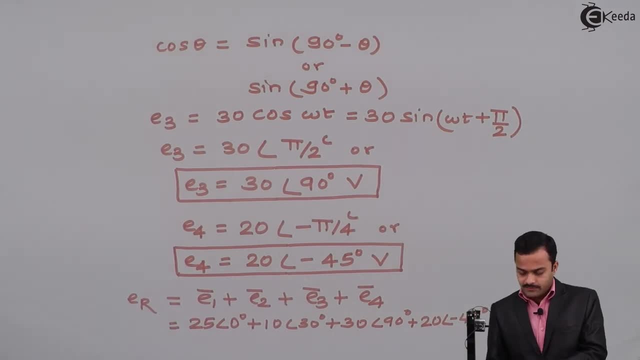 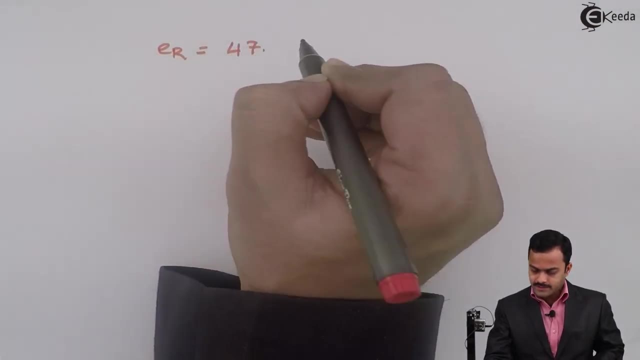 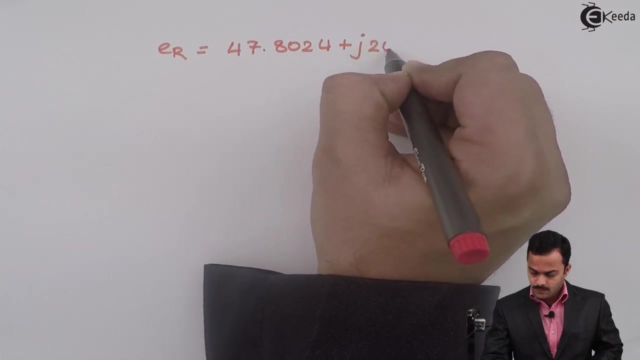 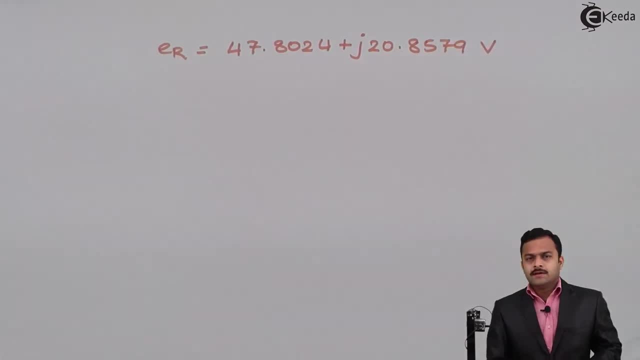 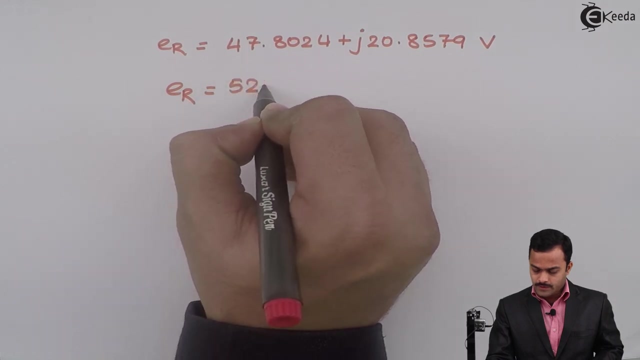 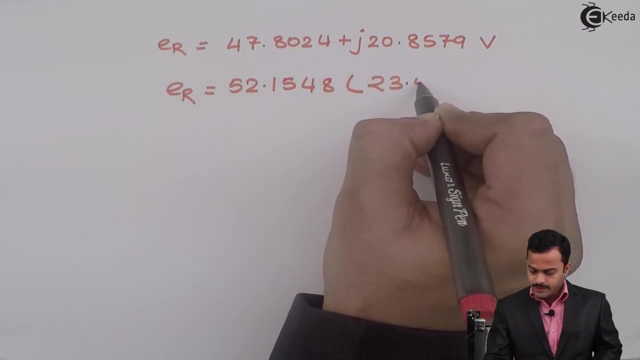 So this will be e are of this angle. Now, how can we estimate resultant Er? So here, Estefive ность A7N0V is $6,478.7.. It is a complex quantity, real part and imaginary part, but what we want in polar form. So in polar form I will get Er as 52.1548 at an angle 23.57 degree volt. 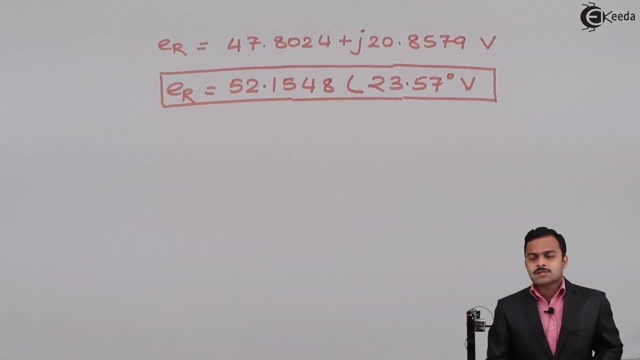 Once you got answer in phasor form it will be very easy to write in a equation form How I can say: E R is nothing, but this is the maximum value, because everywhere we have considered maximum value for E 1,, E 2, E 3 and E 4.. 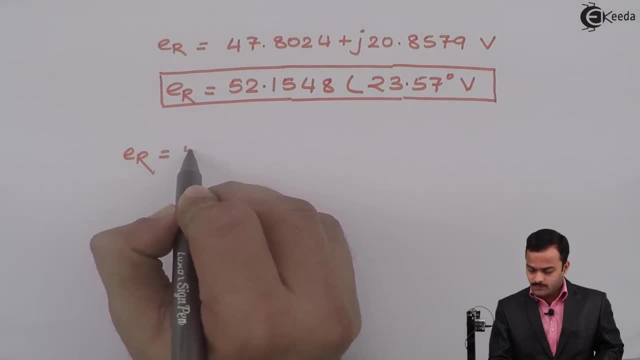 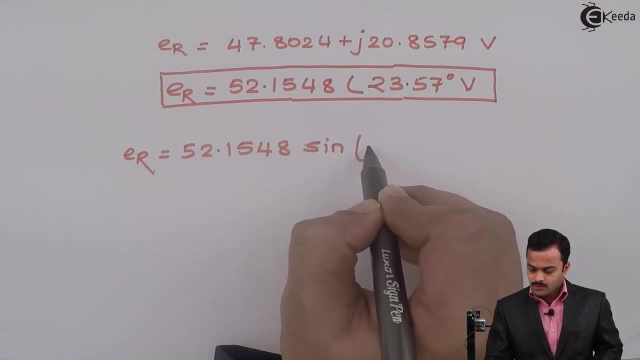 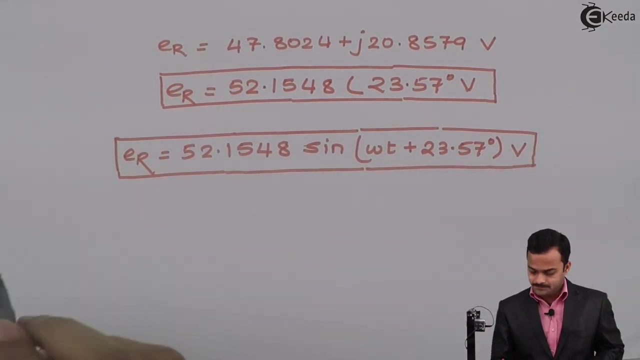 So I can write over here: E R equal to 52.1548 sin, omega, t and angle I am getting over here is positive, So it is a plus 23.57 degree volt. Let us represent all the quantities. This is in phasor diagram.